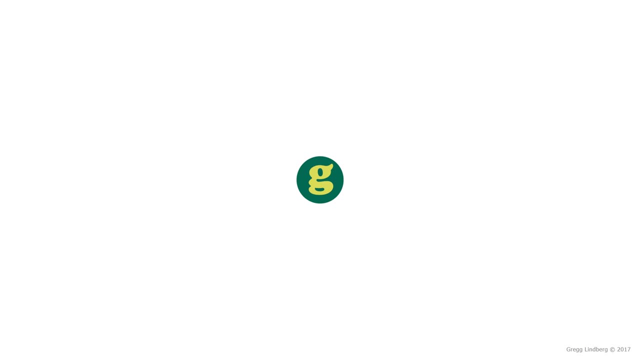 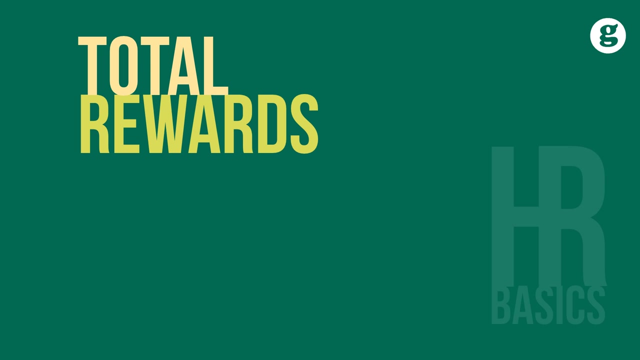 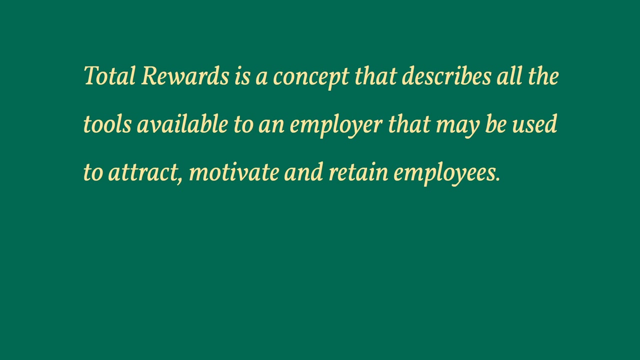 HR Basics is a series of short lessons designed to highlight what you need to know about a particular human resource management topic. In today's HR Basics, we define total rewards and explore the total rewards model. Total rewards is a concept that describes all tools available to an employer that may be. 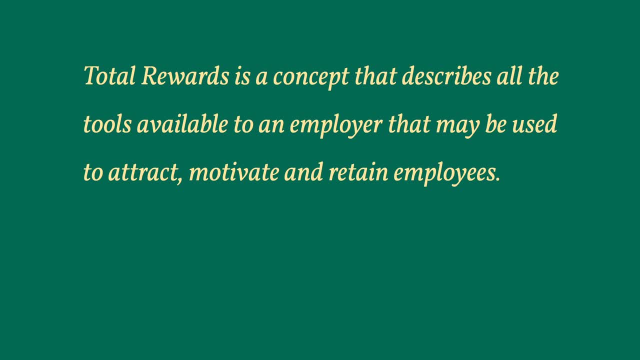 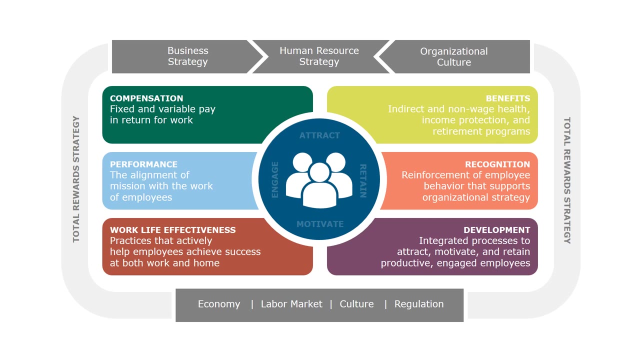 used to attract, retain, motivate and engage employees To an employee or candidate for employment. the notion of total rewards includes perceived value as a result of the employment relationship. Originally introduced by World at Work in 2000,, the total rewards model has evolved to depict the 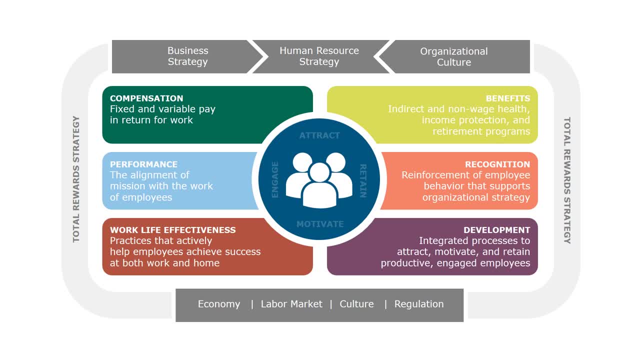 strategic elements of the employer-employee exchange. My total rewards model has been adapted to reflect how external influences impact total rewards strategies and how they affect the overall performance of the employee. It has become clear that the battle for talent involves a highly effective, strategically designed compensation and benefits program. As the concept of total 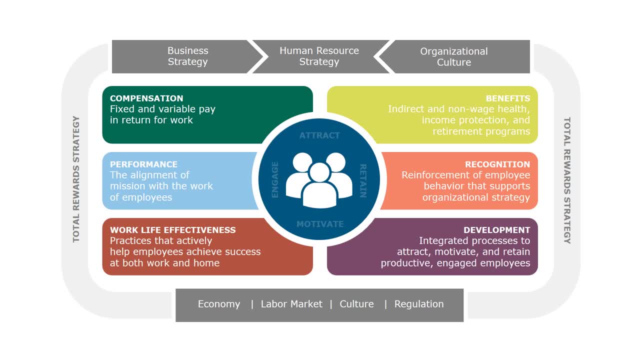 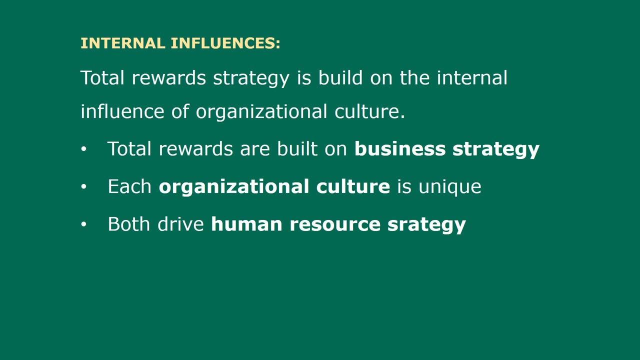 rewards accelerates human resource. professionals must use the total rewards model to take a much broader look at how we attract, motivate and retain employees. HR professionals usually agree that human resource and employee rewards strategies should be based on the organization's business strategy. At the same time, every business has a unique 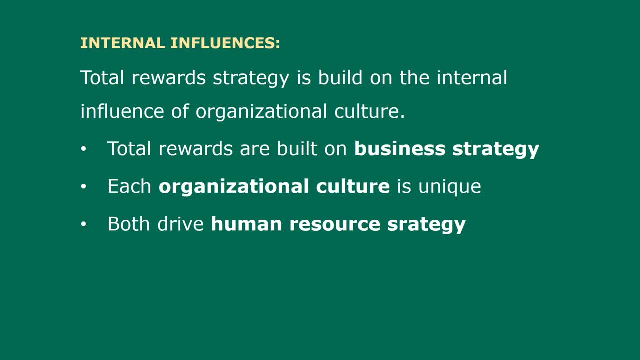 organizational culture that defines how we do things around here. Business strategy and organizational culture drive the design and execution of the approach an organization takes, related to every facet of its human capital or its human resource strategy. In turn, that HR strategy drives the development and 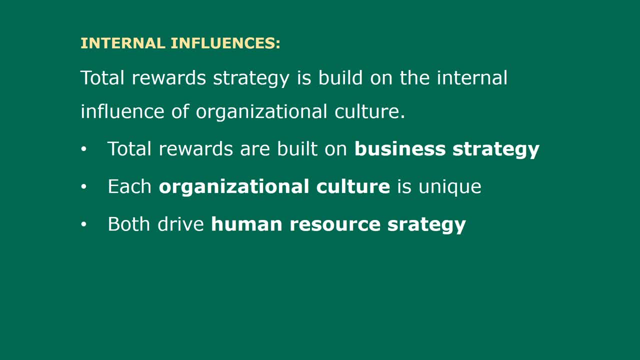 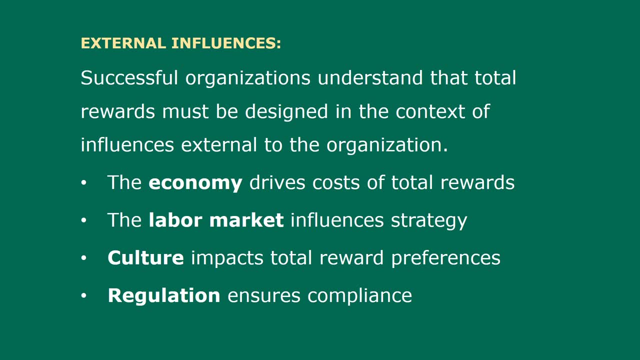 administration of a total reward strategy. Successful organizations understand that total rewards must be designed in the context of influences external to the organization for which there is little control. The global economic landscape has a profound effect on total rewards, especially the costs, which are among the highest. 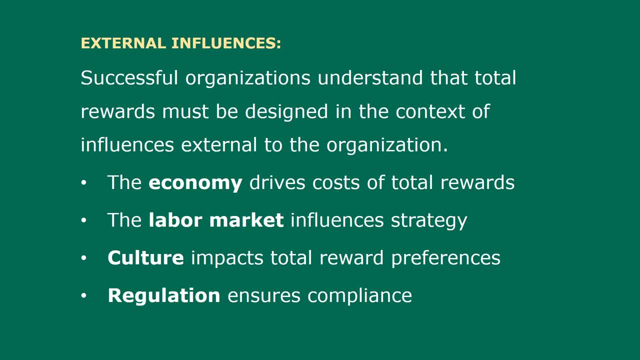 expenses incurred by organizations. Total reward professionals must understand the labor market trends and movements to reach the sweet spot of attracting the necessary talent at a cost that's a little more affordable and sustainable to the organization. Cultural norms and social morals impact employee preferences for different types of rewards. Finally, in the realm of 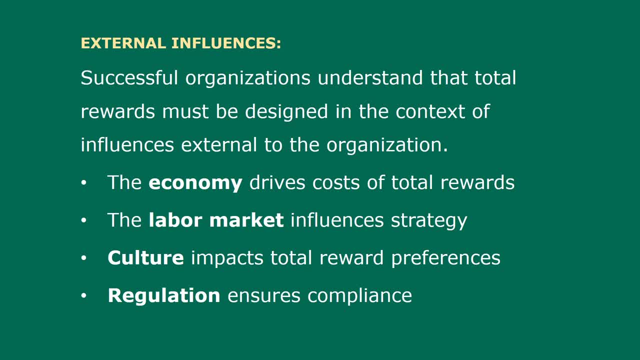 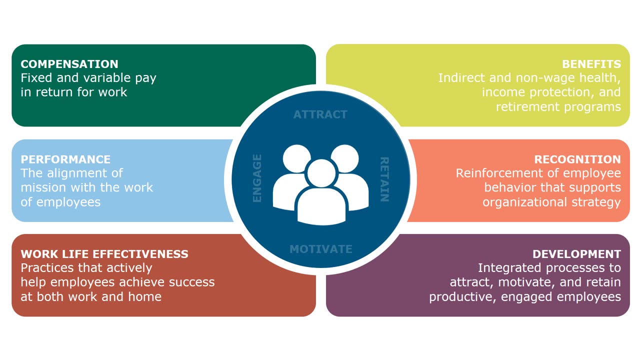 external influences. regulatory issues pertaining to total rewards vary widely and must be well managed by total rewards professionals to ensure compliance. There are six components of a total reward strategy, each of which includes programs, practices, elements and strategies. The first component is the total reward strategy. The 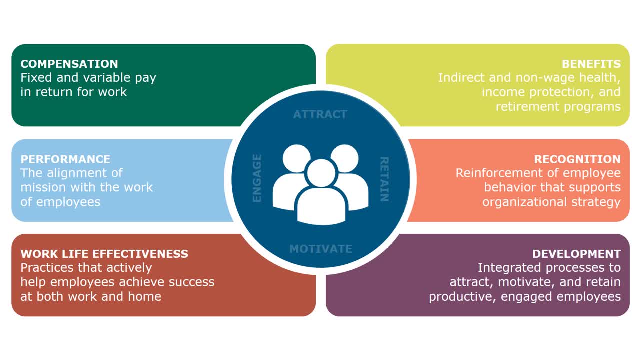 total reward strategy is a system of requirements and dimensions that collectively define an organization's strategy to attract, motivate, retain and engage employees. First, compensation: the fixed and variable pay provided by an employer to its employees in return for work. Second, 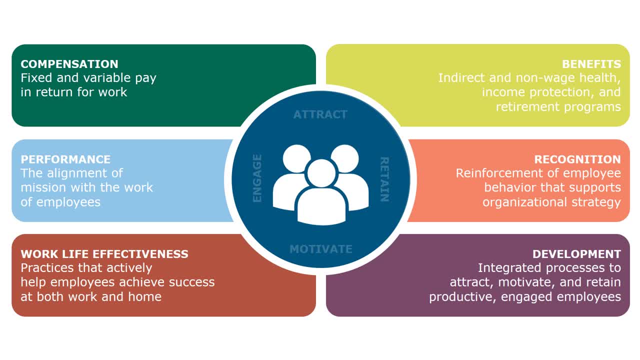 benefits, the indirect and non-wage health, income protection and retirement programs that provide security for employees and their families. Third: performance management: the alignment of organizational mission and the ability to manage the organization's financial and social needs. Third: recognition with the work of employees. Fourth, recognition: reinforcement of employee. 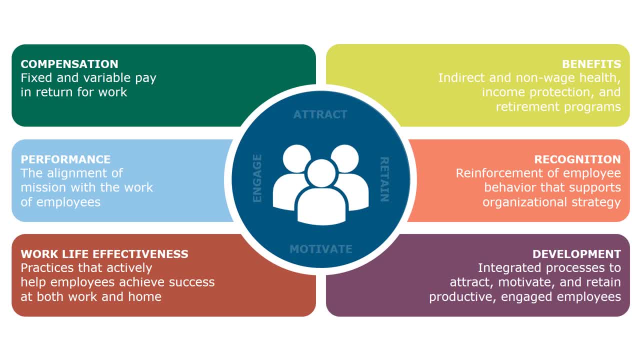 actions, efforts, behaviors or performance that support organizational strategy. Fifth, work-life effectiveness: practices that actively support efforts to help employees achieve success both at work and at home. And sixth and finally, talent development: integrated processes to attract, motivate and retain productive and engaged employees. These elements 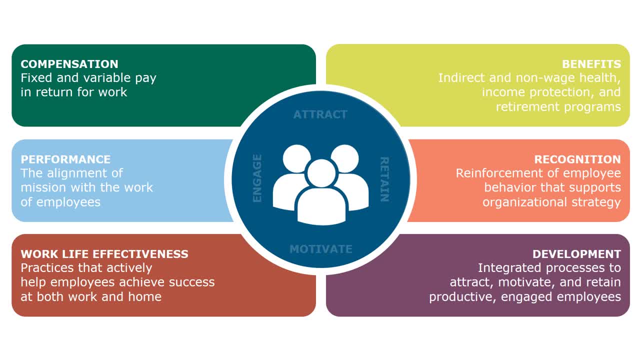 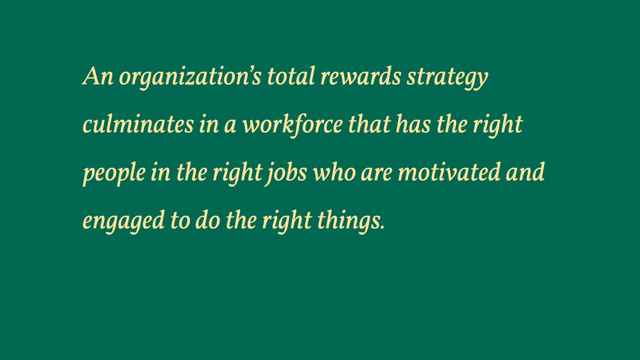 represent the toolkit from which an organization chooses to offer total rewards. The correct combination of these strategies will result in satisfied, engaged and productive employees, who will generate desired organizational outcomes. An organization's total reward strategy culminates in a workforce that has the right people in the right jobs, who are motivated and engaged. 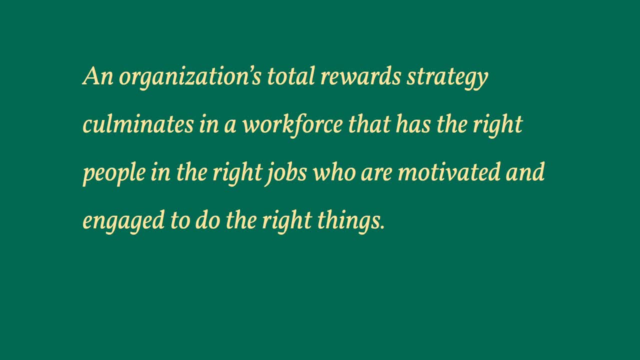 to do the right things. Employees feel loyal to the organization and its success. The model demonstrates the dynamic relationship and exchange between employers and employees, Champion the needs of our employees and our business interests to realize results through engagement.